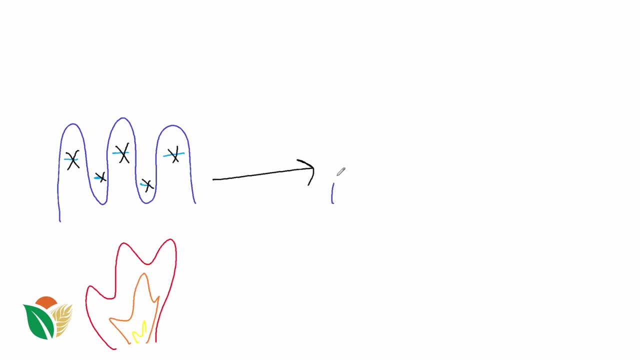 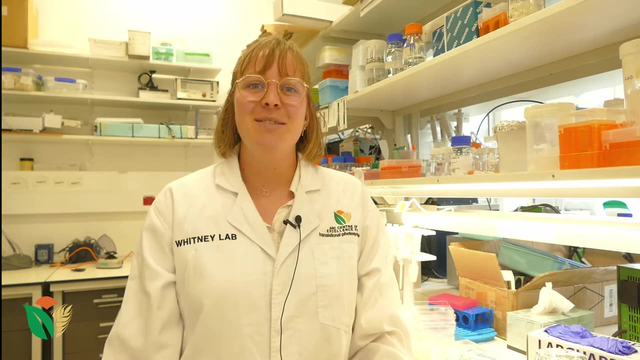 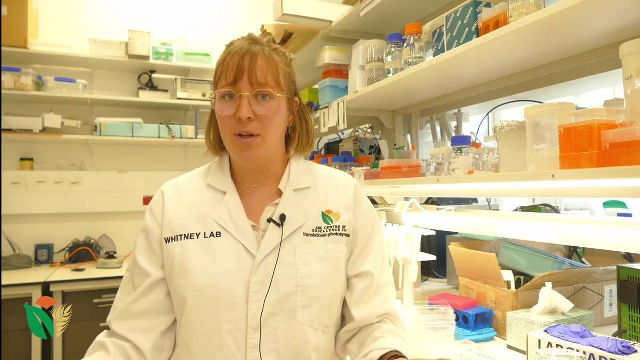 This is called denaturing, And when that happens, they can no longer perform chemical reactions. Chemical reactions in biology are still chemical reactions, And this means that energy in the form of heat makes them go faster. At low temperatures there isn't much energy and things move slowly. reactions go more slowly. 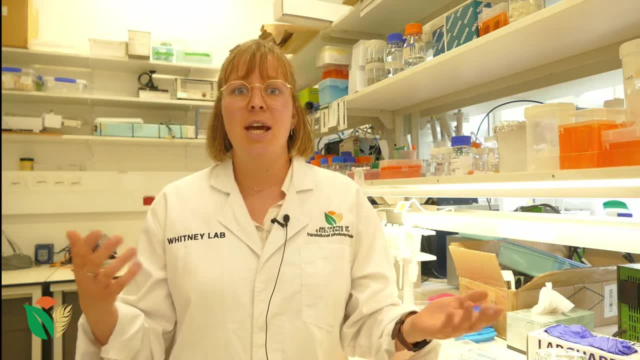 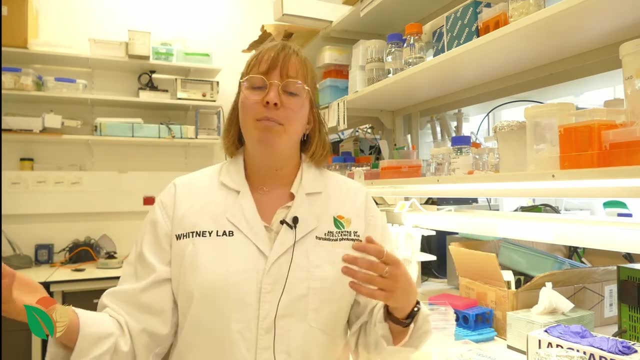 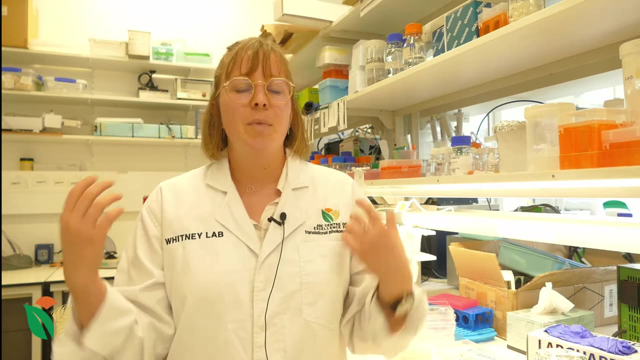 This means that for enzymes, the fastest rate is usually an optimisation between a temperature at which it's warm enough for the substrates and the enzyme to be moving about, but cool enough that the enzyme still maintains its tertiary structure. And because most enzymes are made of proteins, they're sensitive to the same things that proteins are sensitive to. 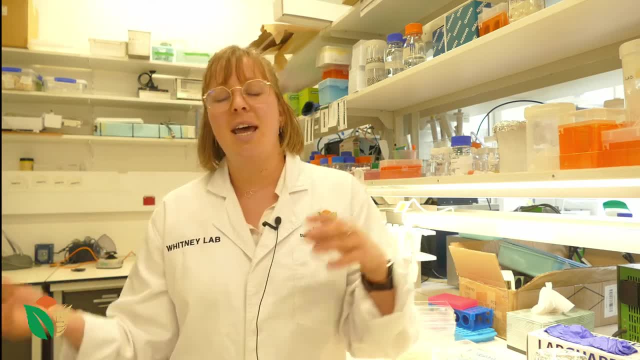 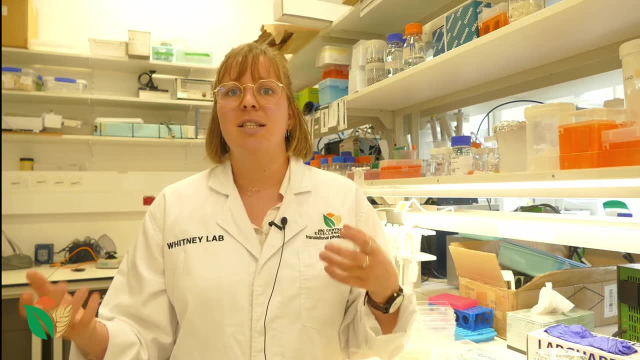 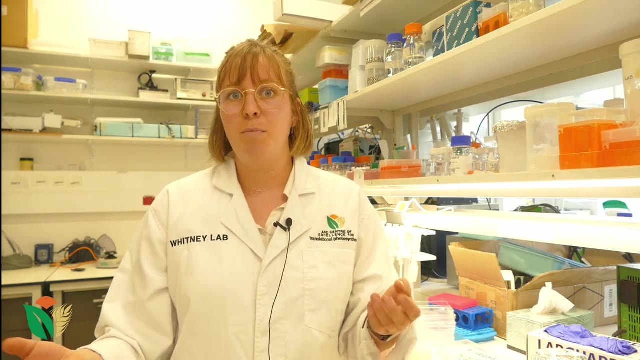 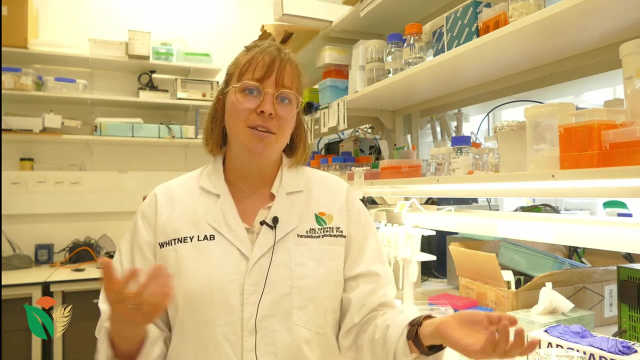 So proteins are made up of amino acids, And each of the 20 amino acids differs by the side chains, And some of these side chains are sensitive to pH. They might change their shape or their charge at different pHs. This has a flow-on effect to the rest of the protein and can result in differences in the way that protein functions. 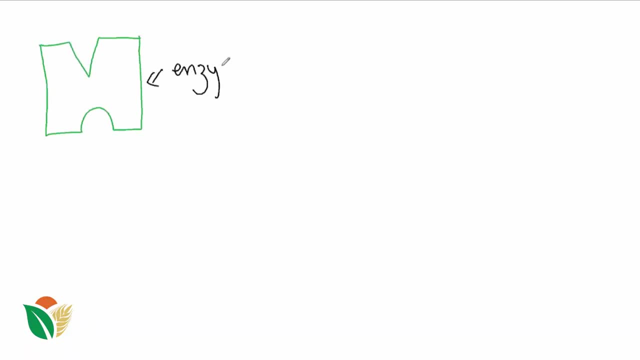 Enzyme activity can also be altered by the presence of other compounds in the solution. it's working in. Competitive inhibition occurs when a substrate similar to a substrate in the form of an amino acid or a substrate of the enzyme is added. This inhibitor also fits nicely into the active site of the protein. 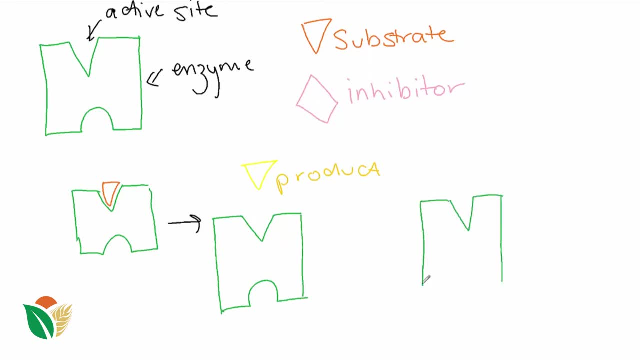 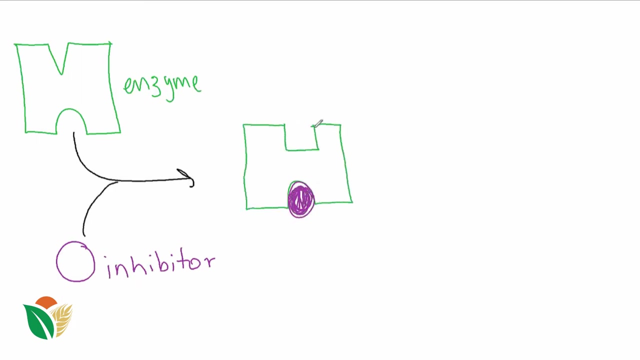 When the non-substrate substance is bound, it prevents the substrate from binding and this reduces the rate of reaction. Non-competitive inhibition occurs when the inhibitor doesn't bind to the active site but to another part of the enzyme. When the inhibitor is bound, the shape of the active site changes and the substrate can no longer bind. This reduces the rate of reaction. Inhibition doesn't only occur by the action of non-substrate substances, though In some cases the presence of large concentrations of the substrate or the product can result in inhibition of the enzyme. High concentrations of the product means that the product is more likely to rebind to the active site than the substrate is. 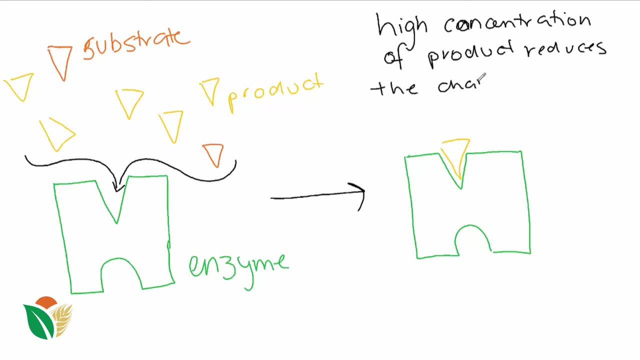 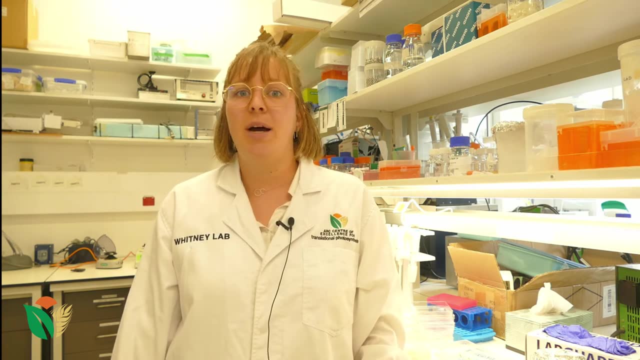 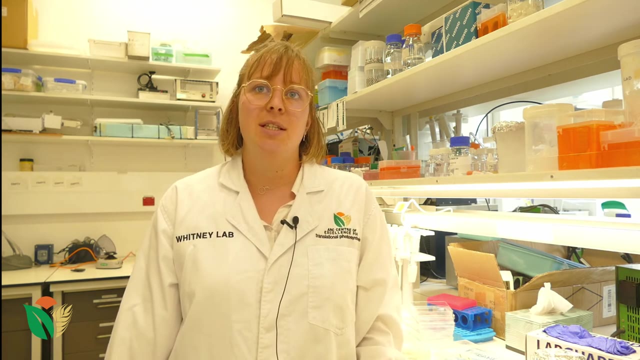 This means that the reactions occur less frequently and the rate of reaction slows. Processes of enzyme inhibition are important biological processes that are closely regulated within organisms. Rubisco is a really important enzyme in photosynthesis. It's the enzyme in plants that fixes carbon dioxide from the atmosphere.